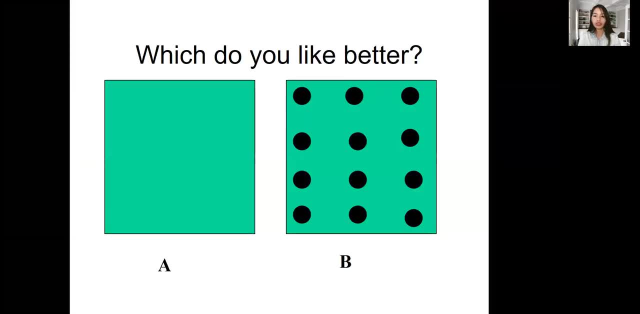 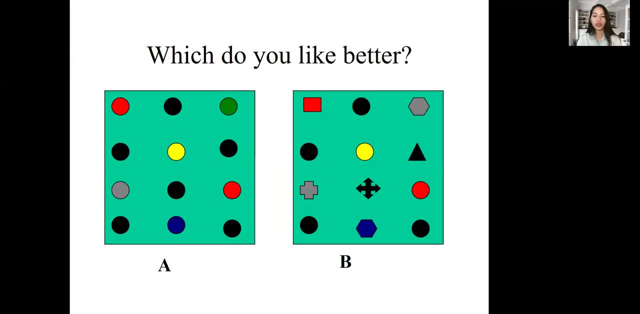 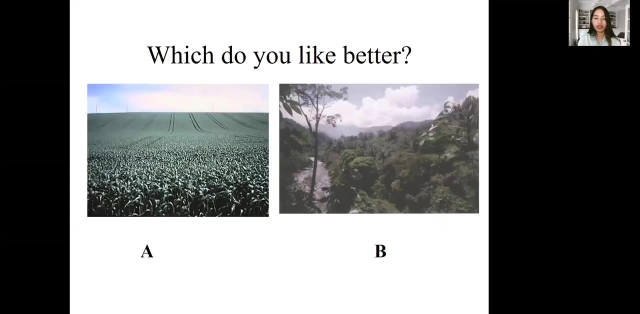 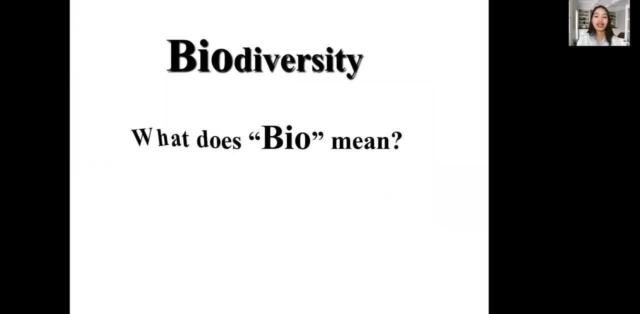 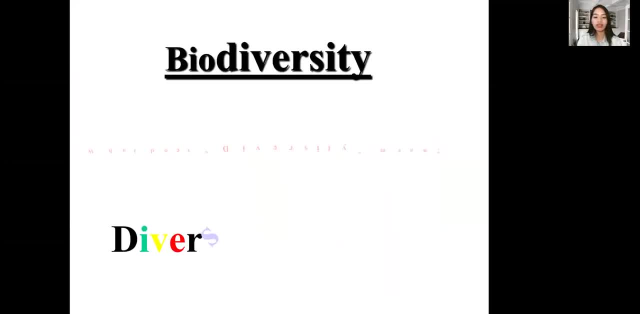 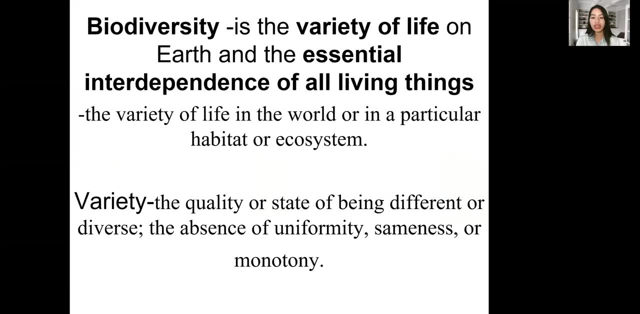 How about the diversity? Diversity is the variety, It is the variety or the quality of a state Being different, Being different from another organization. Uniqueness It is not close, It is not in réussite. There's a variety, so it's unique, being different or diverse. 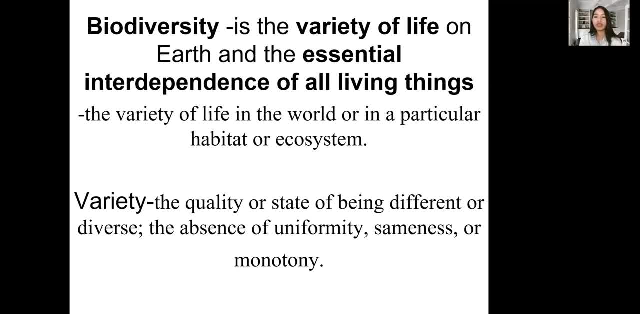 So biodiversity? you can already define what is biodiversity: It's the variety of life on Earth and the essential interdependence of all living things. So our biodiversity is: we are interdependent, Our organisms in ecosystem is interdependent. Another definition: the variety of life in the world or in a particular habitat or ecosystem. 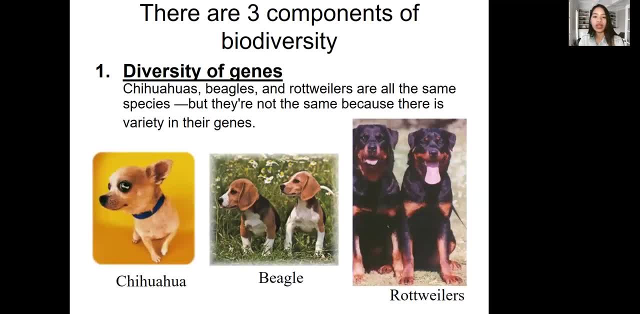 So that is biodiversity. There are three components of biodiversity. First is the diversity of genes. What is this diversity of genes? Example of that is Chihuahua, Beagles and Rattlers are all the same species. They are all the same dog. 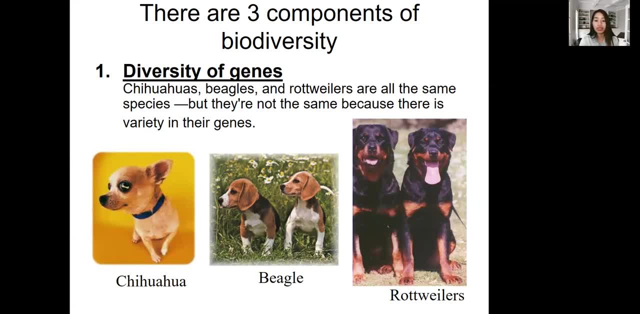 But they are not the same, because there is a variety of genes. There is a variety in their genes. So the genes of Chihuahua are different. The genes of Beagles are different. The genes of Rattlers are different. 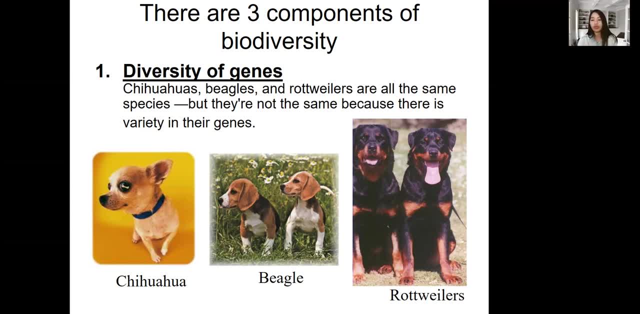 So, as the same as our people, we are all different, We are all human, But then you have different genes. You have different genes from your neighbors, from your friends, And so the diversity of genes. Another example of that is cats. 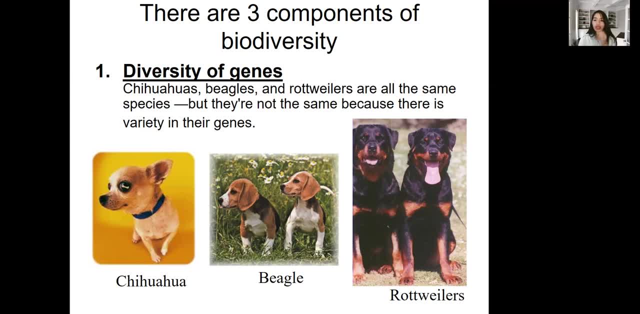 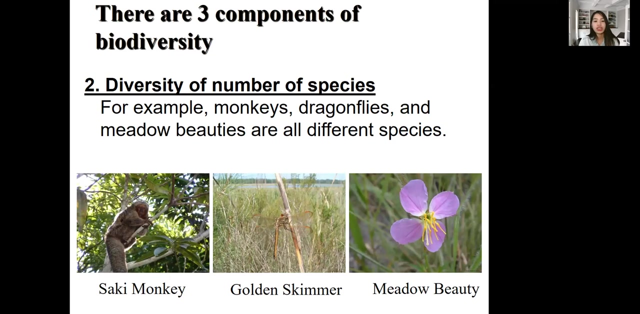 There are different kinds of cats, There are different breeds, So they have different genes And you can cite an example of diversity of genes: The genes are different but the same in their species. Next is the diversity of number of species. Example of that is cats. 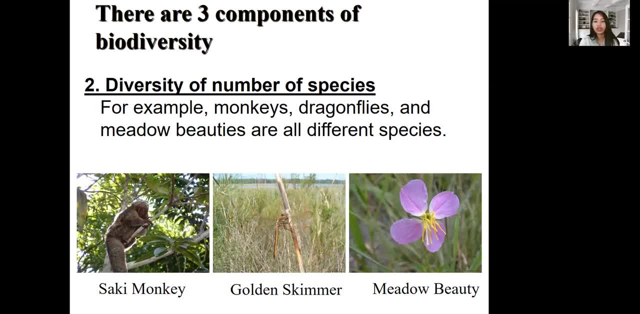 So all of that is monkeys, dragonflies and meadow beauties are all different species. So they are all different species in an area, and then the number of species is different. The population of the monkey is different. The population of golden skimmer is different as well. 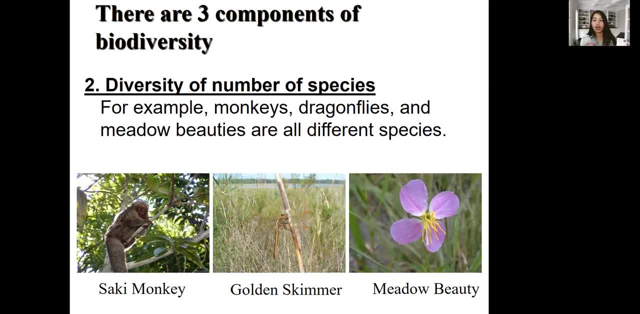 And then the meadow beauty is also different: 90 in the area and then another 90 golden skimmer in area and then 90 middle beauty. so there are different number of species. so, for example, the population of zebra and the population of giraffe is not the same. 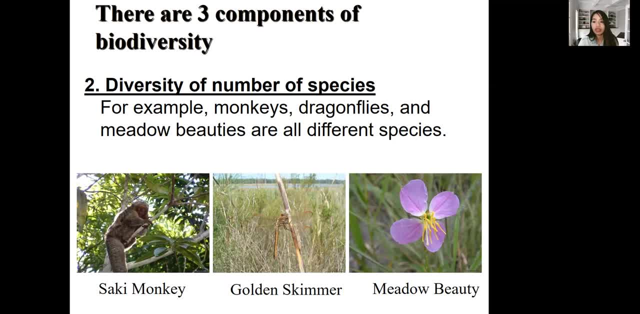 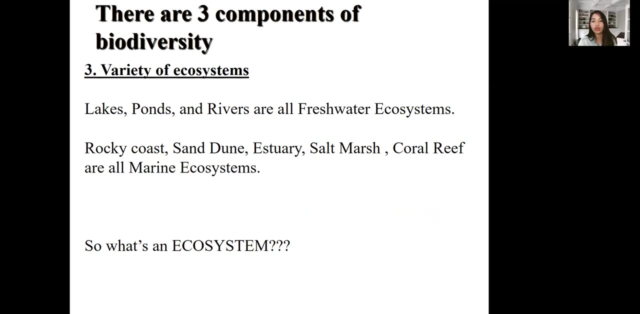 so with the and also with the turtles, monkeys, they have a different population. that is, uh, the diversity of number of species, number, species area. okay, do you understand? next is the variety of ecosystem. so we have already discussed, you already know what it's an ecosystem, so ecosystem is. 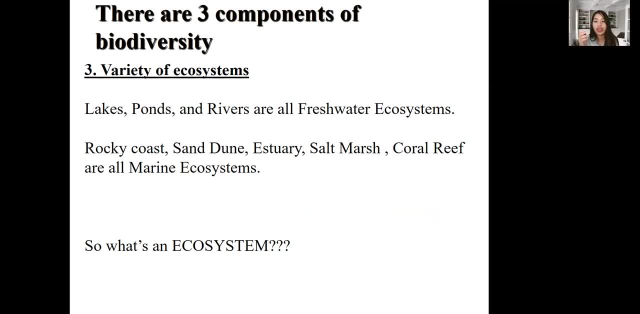 population, different population, community, and then including uh abiotic factors. abiotic factors is the non-layering things, so the variety of ecosystems. so there are different ecosystems here, uh on earth. an example of that is lakes, hands, rivers, fresh water ecosystem. so the life in lakes is not. 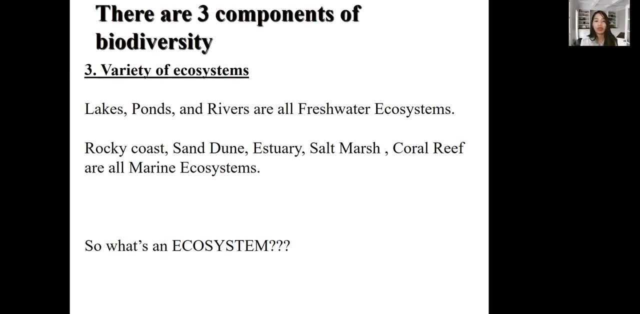 the same in pants, so leaks one of the ways, uh, um, um fresh water. so there is that variety of ecosystem, so different ecosystem. i don't know how um reach our life because, uh, earth, yeah, so it was an ecosystem. so you all already know about that. next is the importance of 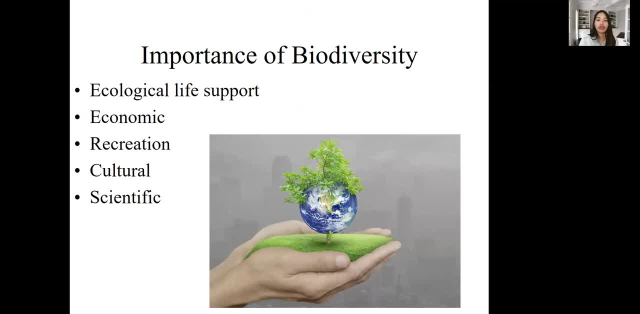 diversity. let's take a look the importance of biodiversity. let's make diversity our life support and the diversity of life and beautiful Eden life support- if it supports that the life of a certain organism, life is now other organizations, supports us. what do we get from our ecosystem? what do we get from our biodiversity? we get oxygen, food. 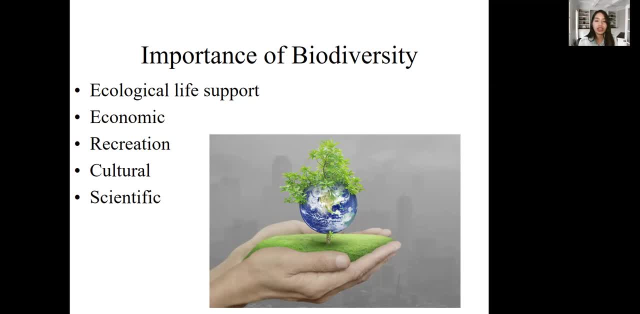 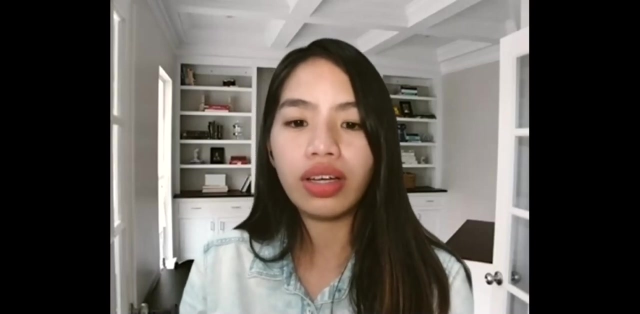 and divine about whirlwiovismonen. life and animalVery, most important thing in this process and then so, which is essential things to mapping ourn new plants? yeah, it supports life. next is economic. when you say economic is the um, what is an ecosystem i mean? so economic is the profit of an uh government. yeah, so. 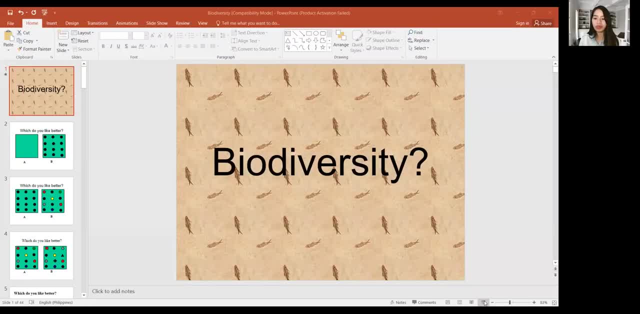 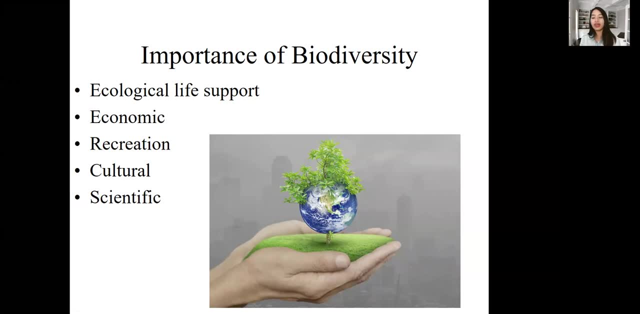 okay, so economic, we get uh uh the uh get benefit from our biodiversity is because of different uh ecosystem. you have a different ecosystem and we get uh a profit from lakes. yeah, so that is the economic. we get profit from our biodiversity, income from our diversity. next is the recreation. 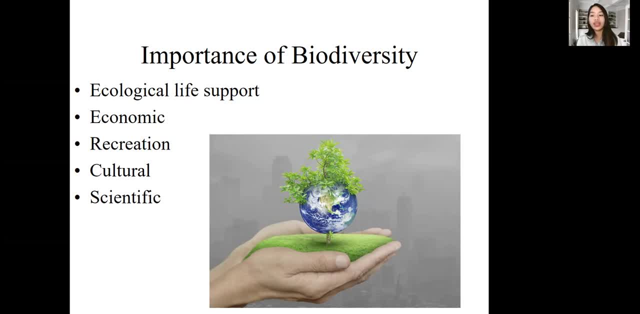 we enjoy lakes, falls, forests. and next is cultural, so there is the preservation of cultures in an area. so there are different. i mean there are areas in the philippines where in there's a certain uh, for example, in baguio, we have our festival instead of being a festival, and 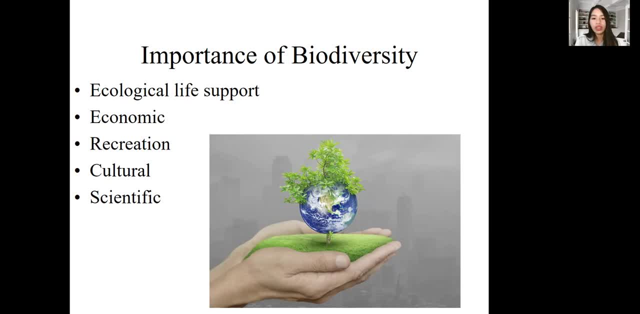 we use different flowers in our festival. so yung mga flowers, paano i-preserve din yung kultur, yung festival na yan. so that is the there's a preservation: biodiversity, preserve our culture. scientific example of that is experiments. ano ba yung mga pinag-experimentan natin? 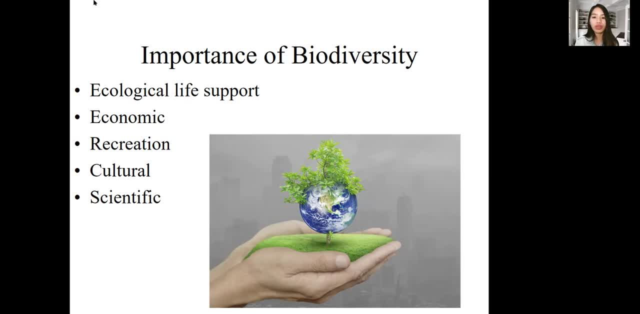 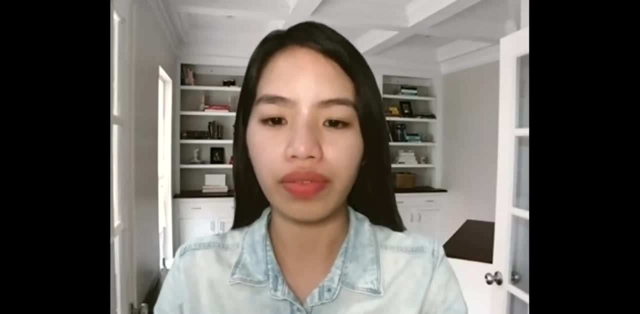 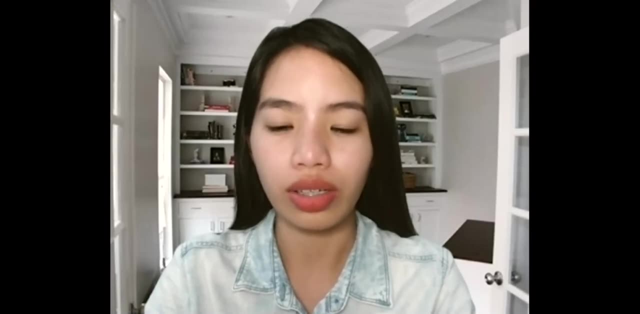 diba yung. so yun yung scientific. another example of that scientific is yung mga cosmetics diba. we get cosmetics from our biodiversity, and then yung mga medicines natin, yung pharmaceuticals yan. so that is how rich our environment lagi ang nakikinabang is. 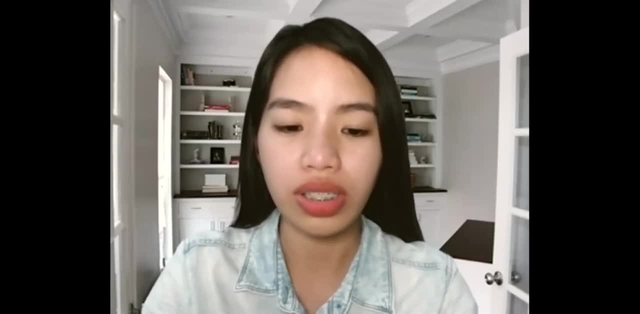 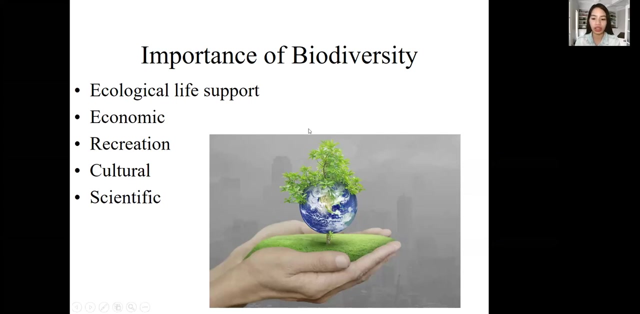 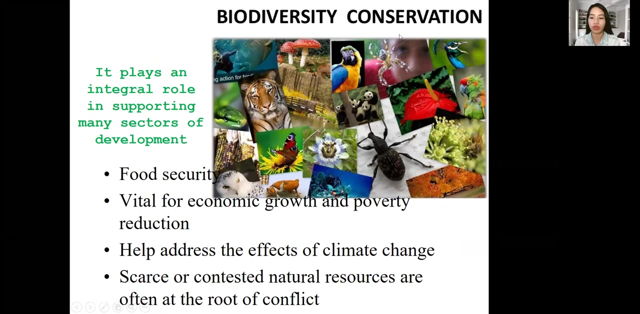 sino tayo, we humans, are always lagi yung nagbe-benefit yan. so next there is all the. there is the importance of biodiversity, so let's move on to the biodiversity conservation. so why do we conserve biodiversity kahit natin kailangan di i-conserve ang mga different lives dito sa earth diba? 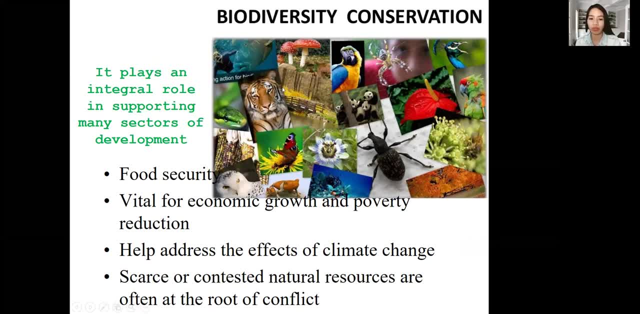 so we need- we need to conserve din yung mga alam kayong paraan how to conserve and then please apply it on your self, on your daily life, kasi a simple act can, it is a big help sa ating ecosystem or sa ating biodiversity. 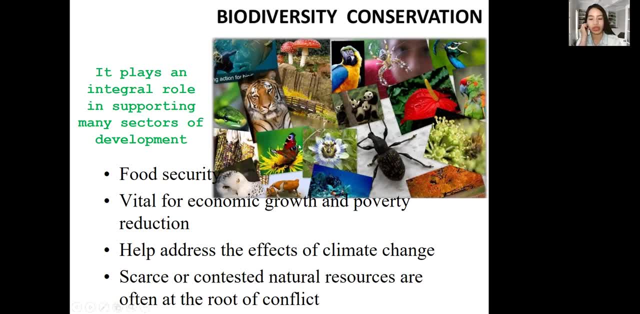 so when you say, when you conserve our biodiversity, we have food security diba, kung maka-conserve lang natin yung mga biodiversity natin, anong food security yan? example, sa mga, sa mga rice diba sa mga fields natin, when we support not only our farmers. 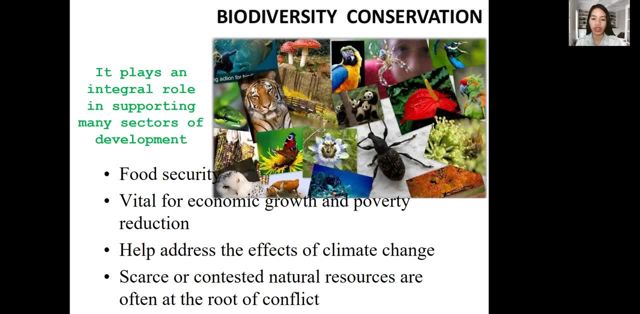 pero yung we support yung farming or fishing, diba may food security tayo doon. when we may yung mga conversions ng mga rice fields into a subdivision, diba nakakita niyo yung effect nya diba. so when we conserve our biodiversity, 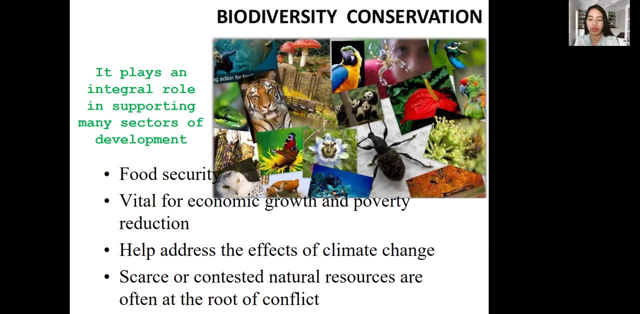 we have food security when we conserve our biodiversity is example of that is dito sa Palawan is the main livelihood also ng Palawan is fishing diba. so there are times na we don't fish yung mga pusit diba, yung mga time na hindi. 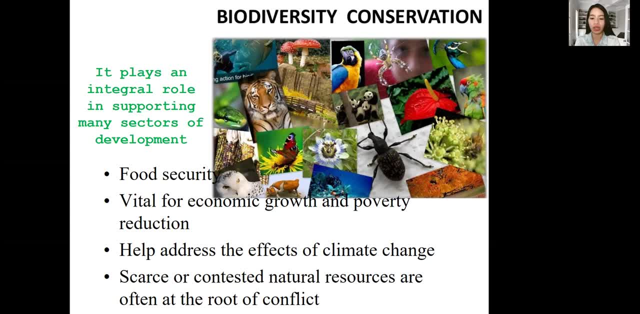 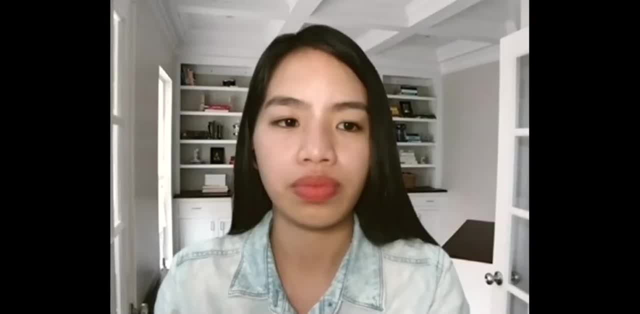 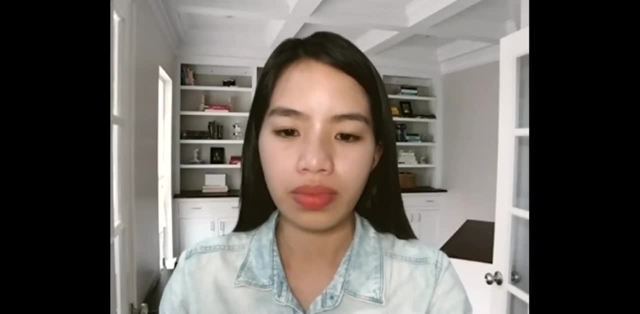 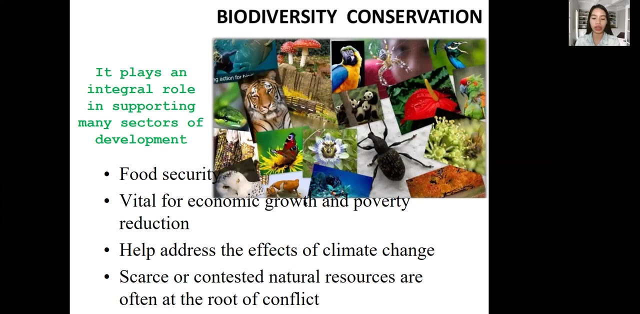 pwedeng i mag fishing para i para may time din sila para magreproduce, so that is a good thing. so the food security next is vital for economic growth and poverty reduction. syempre diba kanina, yung nakita natin yung importance of biodiversity. 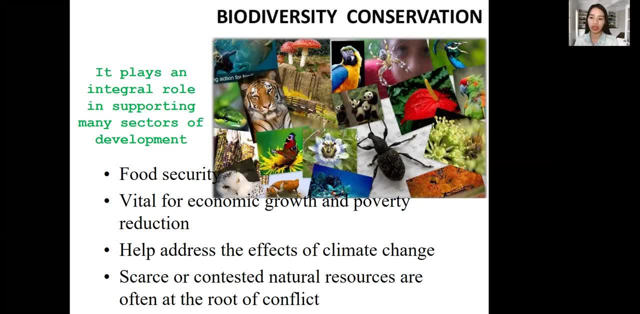 so when we conserve our biodiversity, our different lives, is syempre may economic growth diba. when we use effectively yung mga or properly yung mga ating resources, is syempre may economic growth diba. so yung poverty reduction also. so dito sa koron is yung fishing diba. 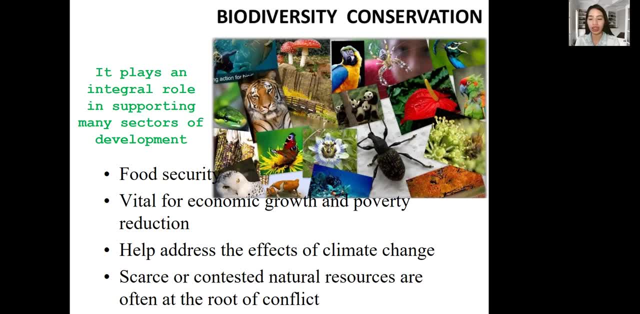 if yung poverty reduction is nakikita natin. nung nawala yung turisan dito, ano nangyari diba? you see how important talaga to conserve yung ating biodiversity. next is help address the effects of climate change. syempre. 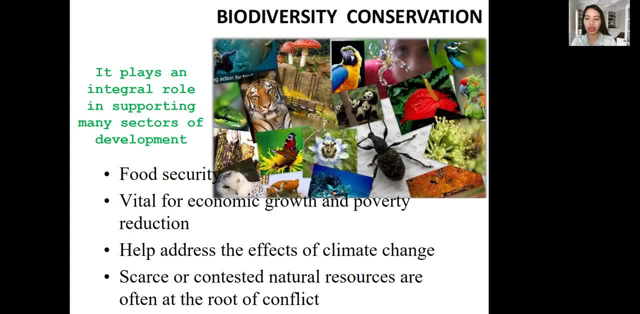 climate change. ano bang panagusapan natin pag climate change? diba pag syempre pag nakonserve ang ating biodiversity. is it help address our climatic, our climate change? and next is scarce or contested natural resources are often the root of conflict, so diba. 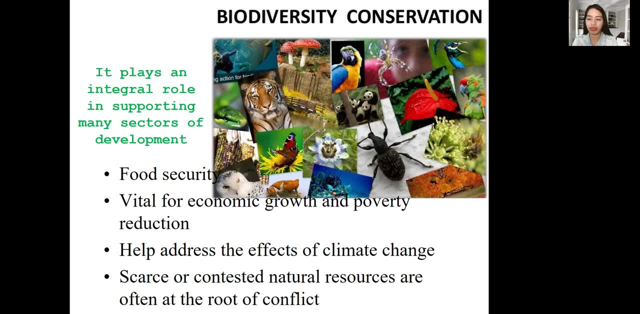 root of conflict talaga ang biodiversity natin, so different LGUs is nakatalo din sila para sa isang resources diba. example of that is Philippines and China, yung pinag-aawaya nila, or yung pinag-aagawa nila. 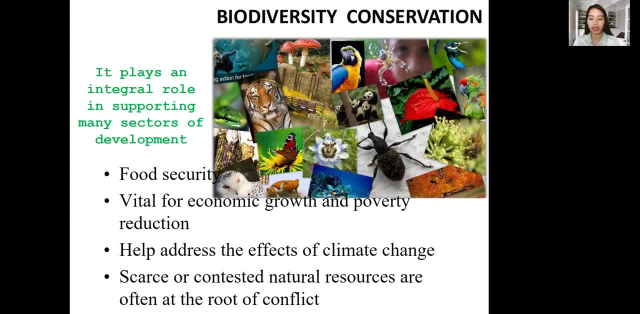 is yung Spratly diba. so when, when we conserve or kung pa, kung ang motive lang natin is pangalagaan diba is sa walang, walang conflict. pero pag yung angking na diba, yun na yung. 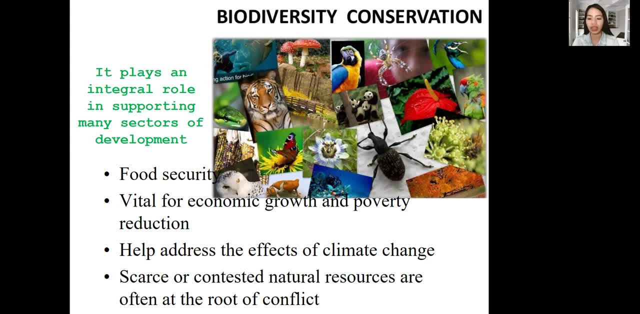 magkakaroon ng conflict. but sa atin diba we need to. yung motive natin is to pangalagaan, to conserve our biodiversity, hindi yung abusuhin diba. we have benefit from our biodiversity. tapos anong yung gagawin natin? 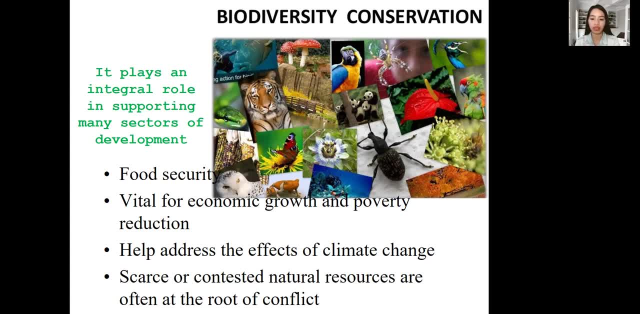 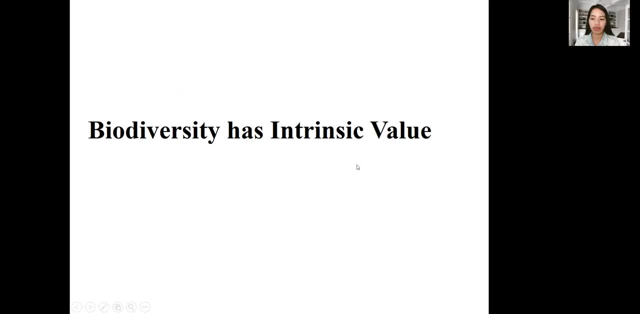 na abusuhin natin diba yun next, biodiversity has its intrinsic value, so all life on earth has value in and of itself. so lagay yung tatayin yung. everything has a value, especially students, and sa akin din, we have value. 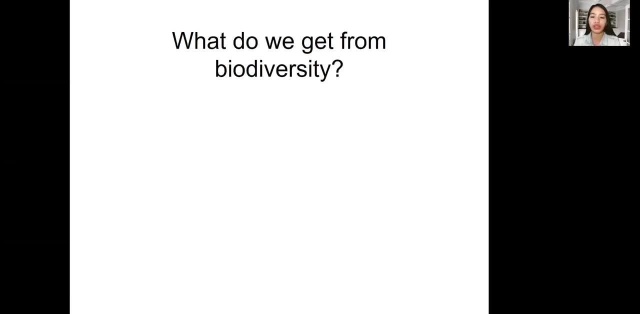 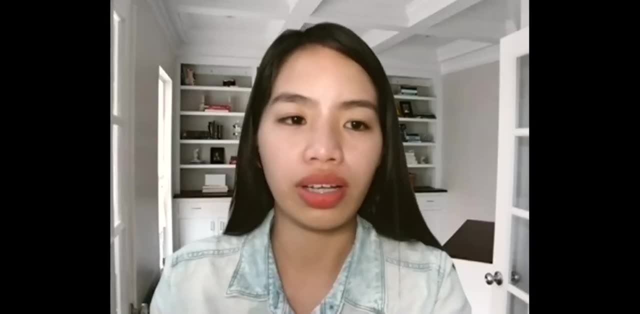 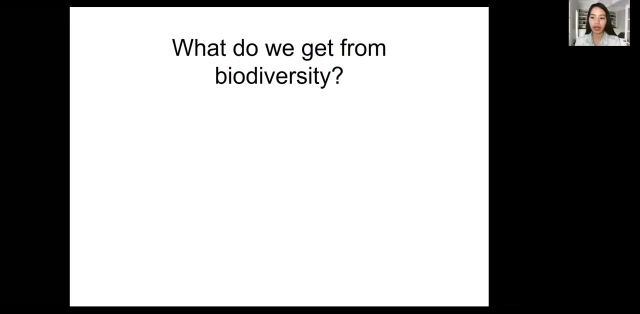 so what do we get from our biodiversity? syempre alam na natin yan lang. so what do we get from our biodiversity diba alam na natin lahat yan? we saw the importance of our biodiversity diba alam na natin lahat yan. 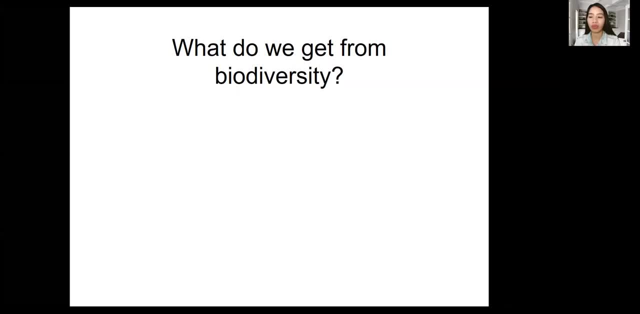 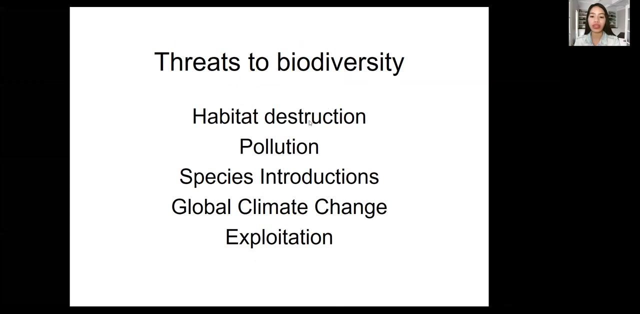 we saw the importance, yung importance, yung conservation. this is oxygen, syempre oxygen, diba, food, clean water, medicine, aesthetics and ideas. so, judged by diversity, habitat destruction, yung pagkasira na kanila, ang mga habitat pollution. example of that is air pollution, water pollution. 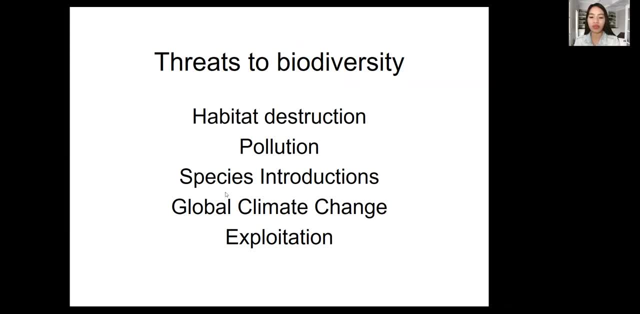 land pollution. species introduction. when we say species introduction is pag nag-introduce ka ng isang species within an area, and especially kung nung binintroduce mo is mas malakas. an example of that is within an area ang mga animals dun is mga. 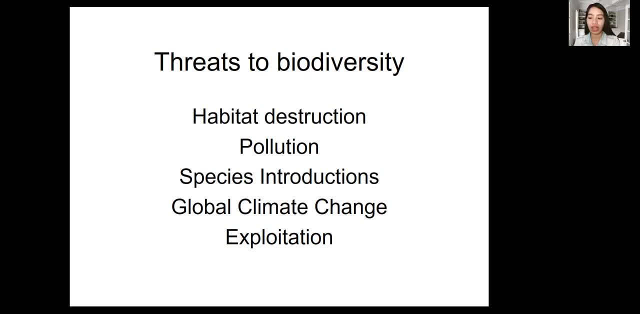 herbivores and then biglahang nagintroduce ng lion, mga ganyan. so ano mangyayari is either yung mababawasan or mamamatay, syempre yung mga herbivore, kasi pwede syang kainin. 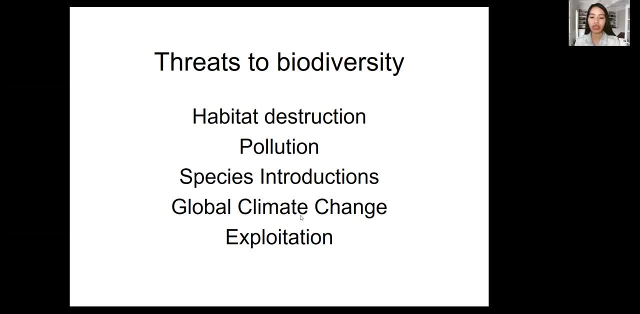 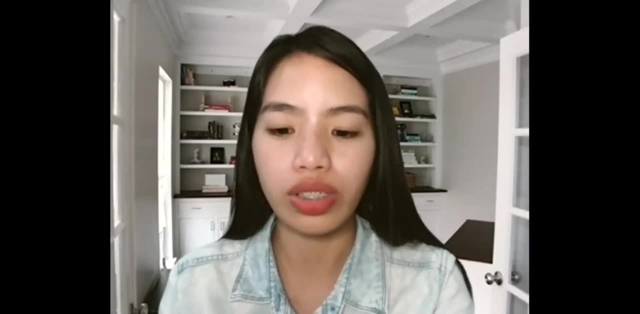 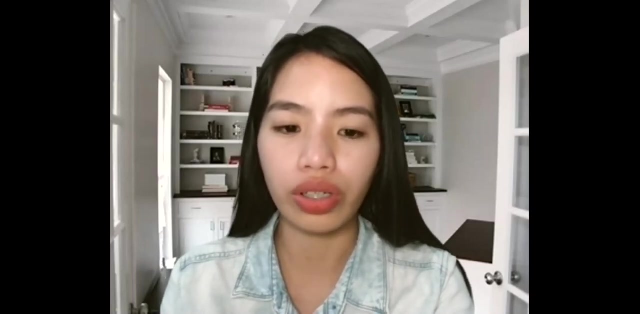 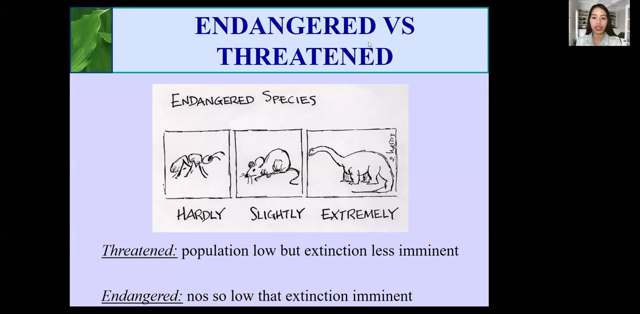 ng lions and so species introduction, global climate change and other types of biodiversity. and the exploitation. what is exploitation class? so this is the using of resources. pag inabuso natin, yung over exploitation is a threat for the biodiversity. okay, next is endangered versus threatened. so threatened.